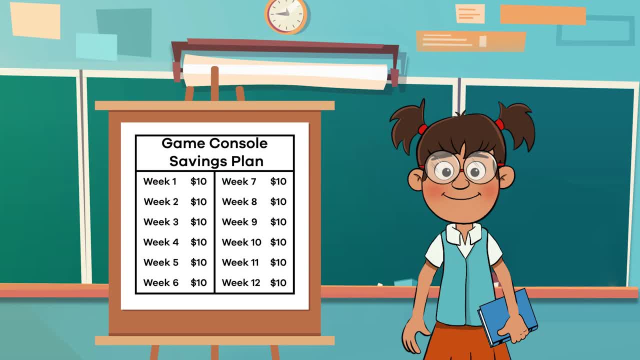 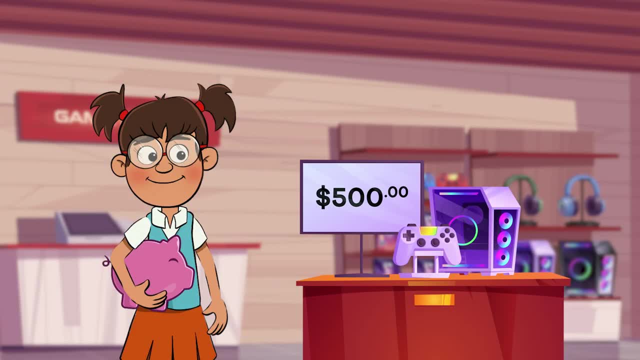 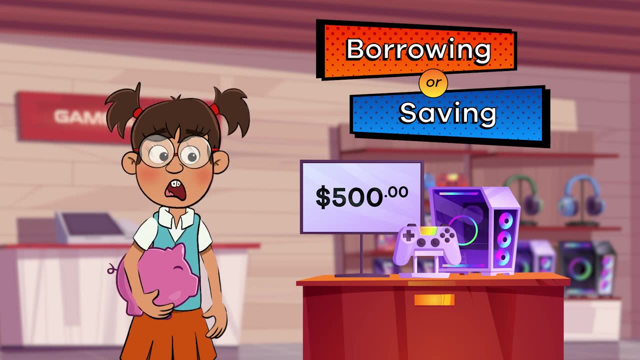 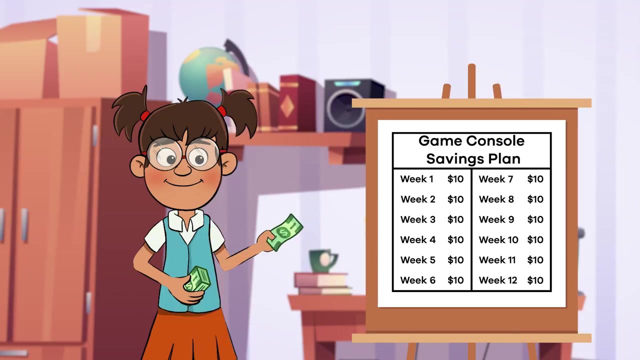 account at a bank. Creating a savings plan is a great idea if you want to buy something. Let's help our friend Frankie Finance decide how to buy the new game console. The total cost is $500.. Each week Frankie gets $20 as an allowance, so she decides to save half of that amount. 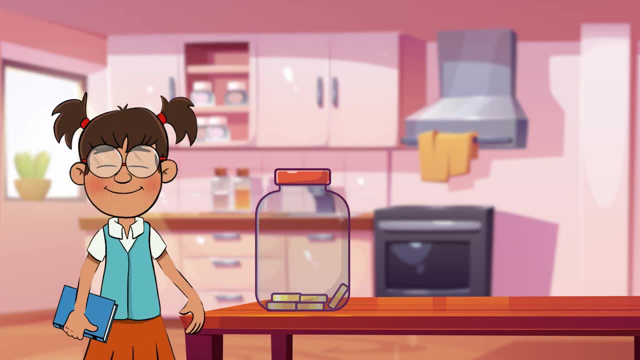 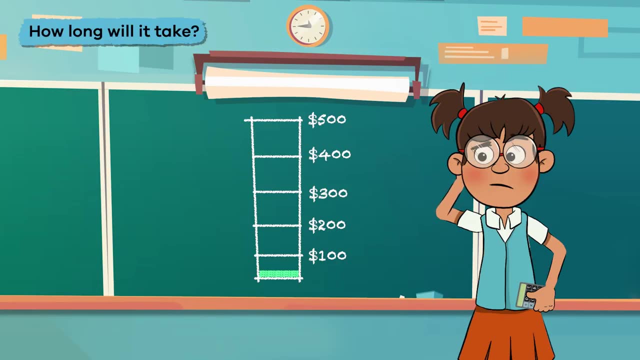 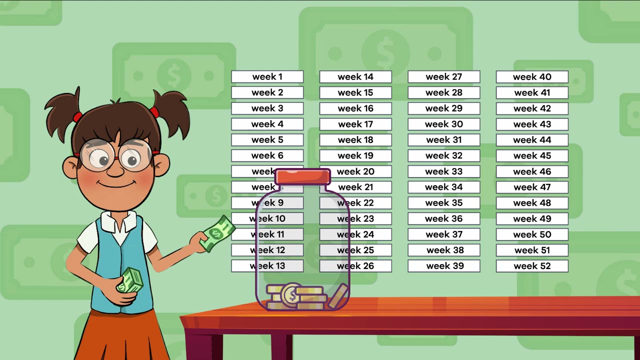 or $10, every week until she has enough money to buy the game console. Let's calculate how long it will take her to save the $500.. There are about 52 weeks in a year. so if Frankie saves $10 per week, it will take her. 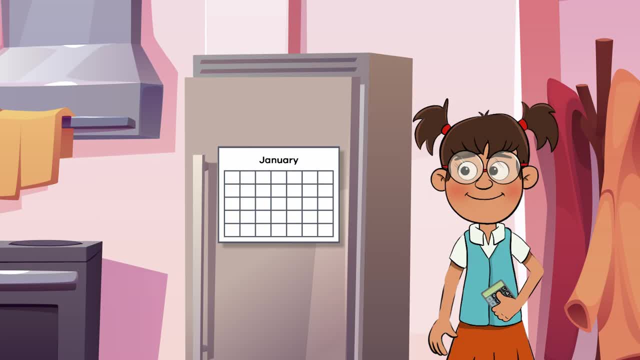 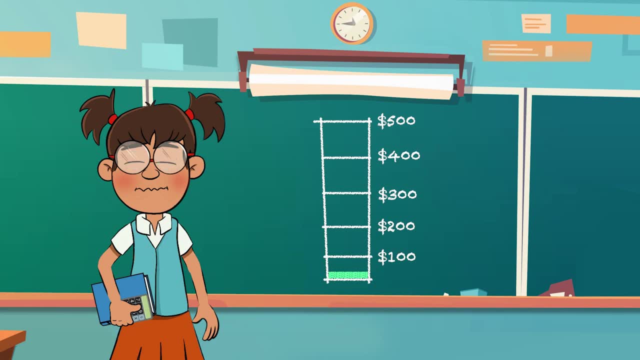 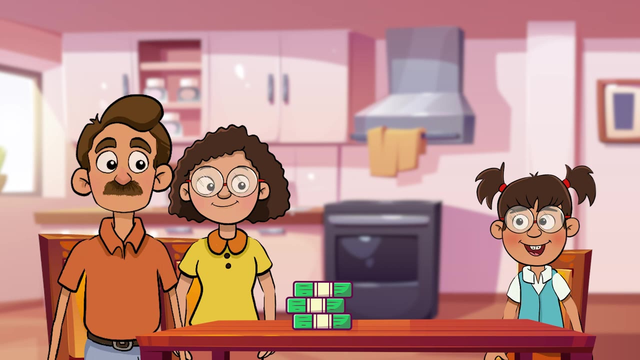 50 weeks to save up enough money. That is almost a whole year of saving. If Frankie does not want to wait that long, she could also borrow the money Her parents offer to be her lender, expecting her to make monthly payments on the loan, The loan payment. 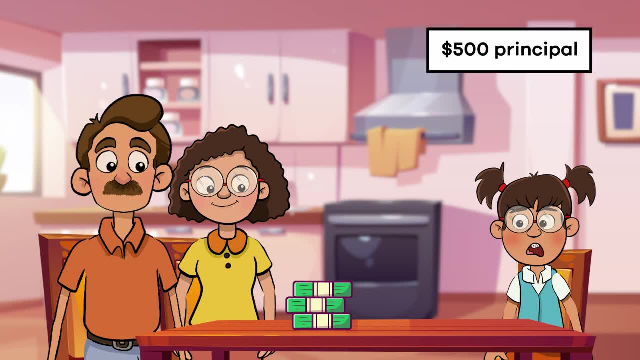 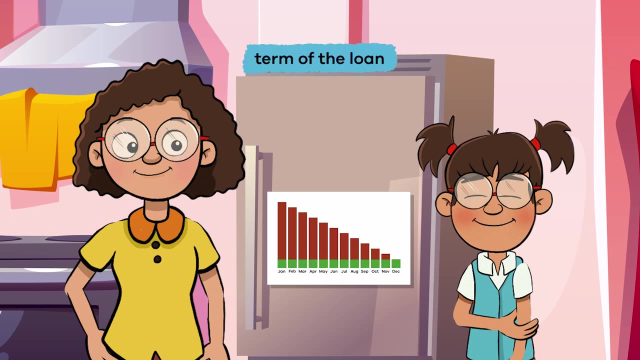 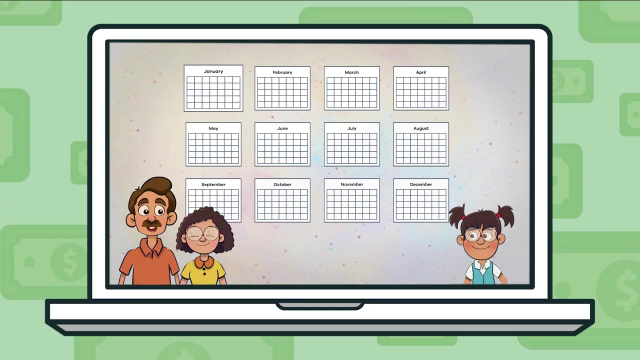 includes the principal or original amount she will borrow, plus interest, which her parents set at 1%. Frankie would also have to make payments to her parents over a specific time period, which is called the term of the loan. Her parents want her to pay back the loan in one year. 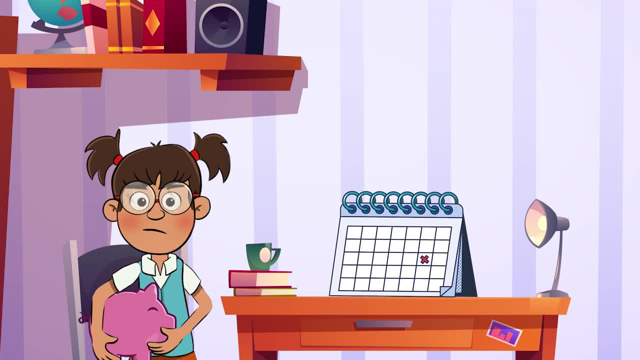 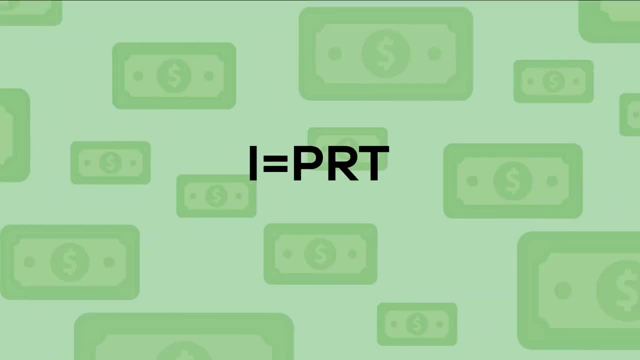 So how much money would Frankie need to pay back exactly? Let's look at this handy mathematical formula to find out. I equals PRT. In other words, interest equals principle times rate, times time. In Frankie's case, this formula would be: 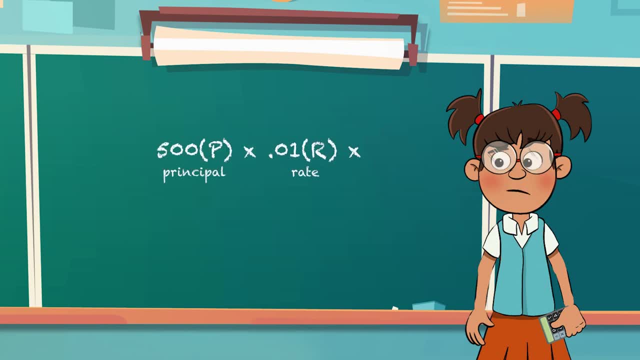 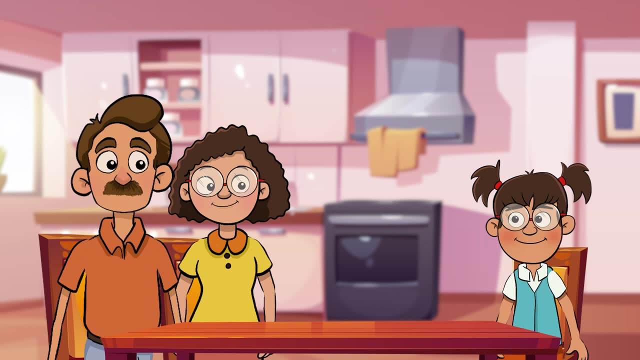 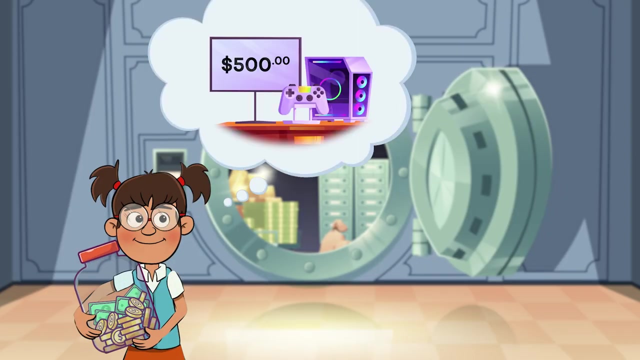 times, which equals $5i. This means that Frankie would need to pay her parents back an amount of $505.. once she adds in the additional cost of interest. What would you do if you were Frankie? Save the money for a year and wait to buy the game console, Or borrow the money to get the console right now.